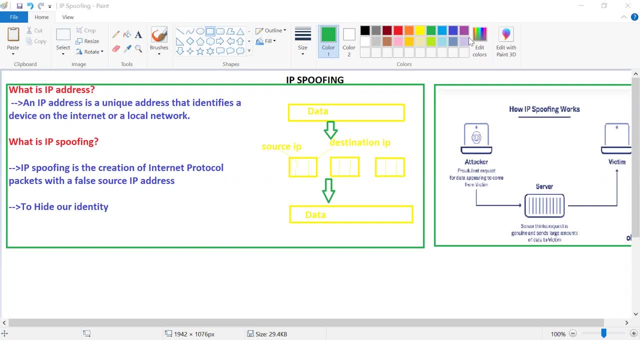 particular device on the internet. So every node on the internet, every device on the internet, is having an IP address. So based on the IP address only we will be identifying a particular IP address, right? Yes, Coming to the IP spoofing guys. what exactly IP spoofing? 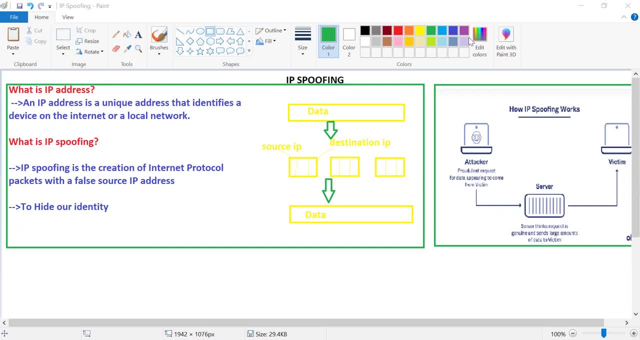 is. we can say that you know simply to hide our identity. to hide our identity, we can say that identity will be using the IP spoofing technique. IP spoofing is the creation of internet protocol packets with a false source IP address. Let's say in general what will. 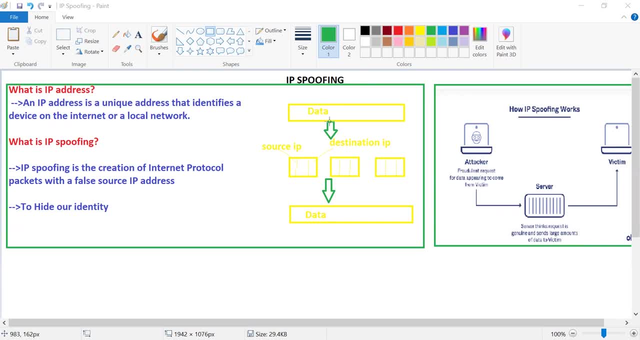 happen whenever you are sending in a data. when you're sending any data, the data will be divided into multiple packets, right? So each packet is having source IP address and destination IP address. Each packet is having source IP address and destination IP address. 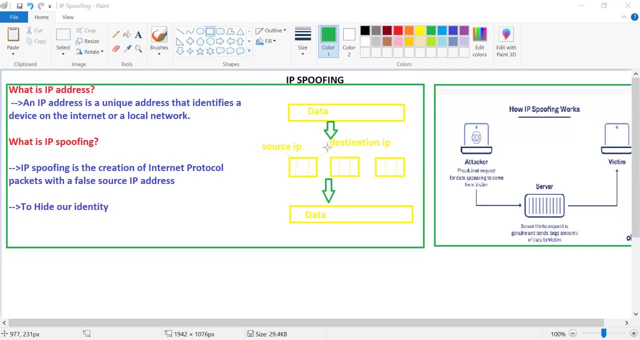 And whenever it is, Whenever it is reaching to the other end, definitely it will be. we can say that it will form into a version format and it will reach to the other end. right, This is a genuine communication. I mean so, whenever you're sending any data, it will be divided into. 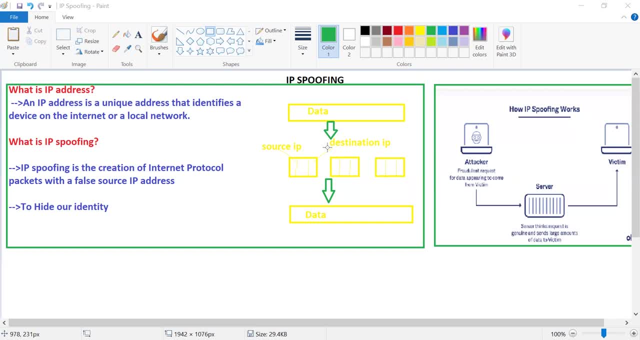 multiple packets. Each packet is having source IP address and destination IP address. This is a genuine communication right. So when you're using IP spoofing now, in IP spoofing we will be changing the source IP address In order to hide our identity. we will be changing the source IP address In order to 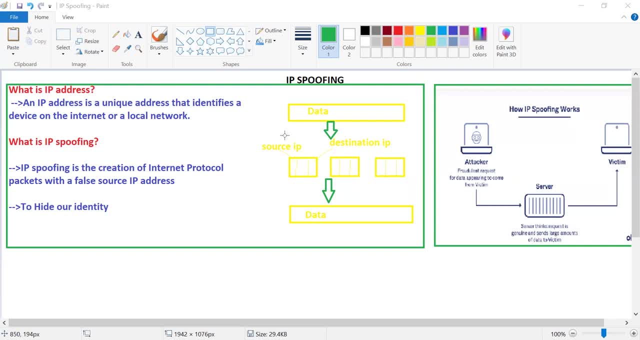 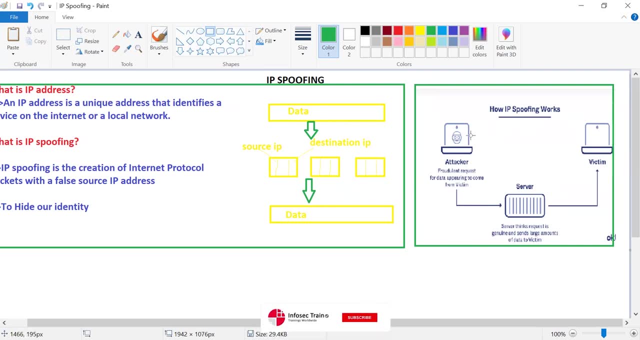 hide our identity. we will be changing the source IP address. Here in its diagram, you can see how IP spoofing works. So, as an attacker, I will spoof my IP and I can create a fake IP address. I can send it to the server and server will think that the request is genuine. 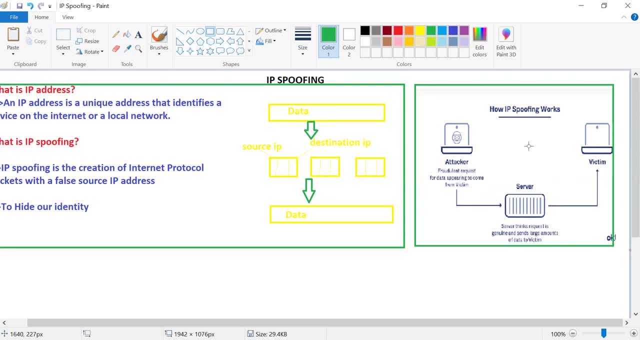 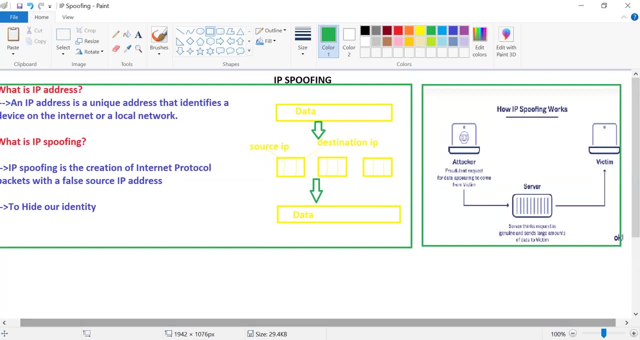 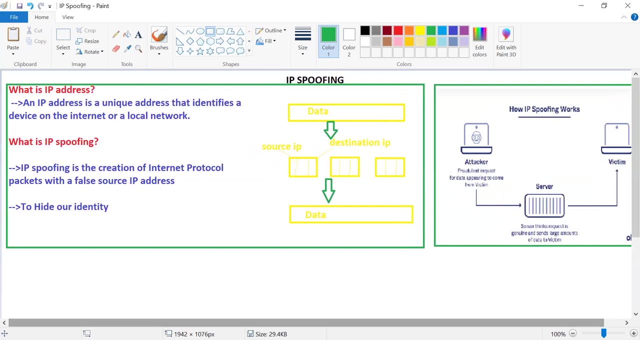 and send large amount of data to the debtor. So this is how spoofing, how IP spoofing works. Okay, IP spoofing- the sounds of man-in-the-middle attacks can happen, DOS attacks can happen and DDoS attacks can happen by using this IP spoofing. 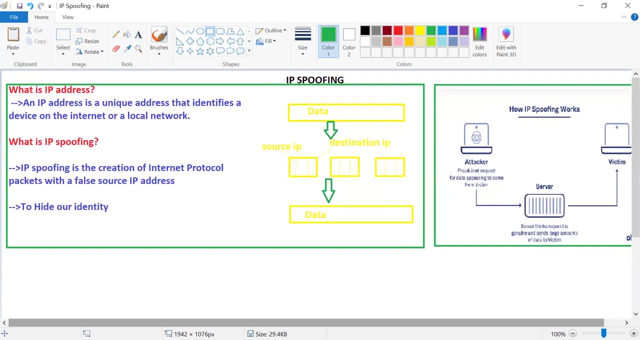 So IP spoofing is basically in order to hide our identity purpose. we'll use the IP spoofing.